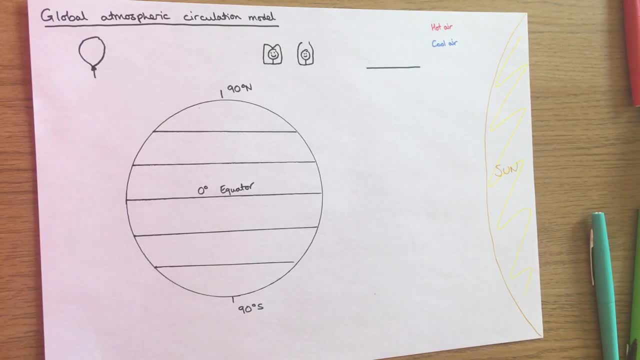 and in turn that affects our climate. it affects where we find different biomes as well. So we're going to go through step by step. it's quite complex, but we'll go through each of the stages. So if you want to draw along with me, you can, or just watch and take it in. First of all, we're 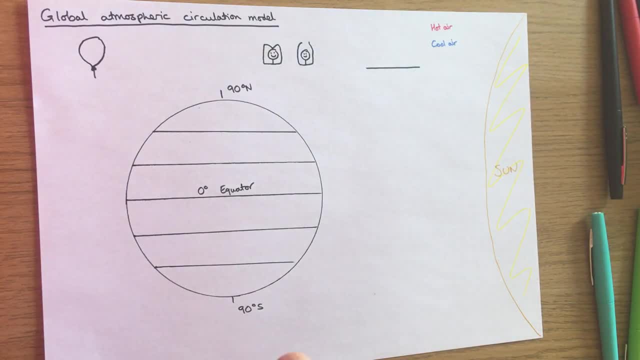 going to have a look at why some parts of the Earth are hotter than others, because clearly we know that the equator is hotter than the poles. So let's have a look at our lines of latitude. first of all, We've got the equator at zero. I've labelled on 90 degrees north and south. Now this: 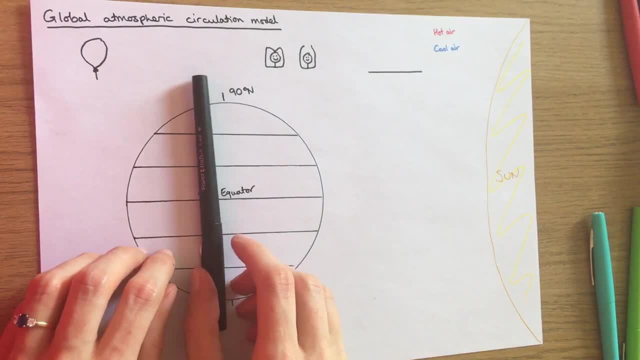 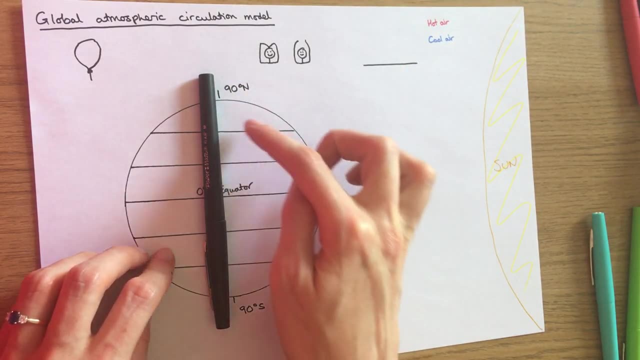 isn't the temperature. this is due to our lines of latitude. so, for example, if I were to draw a line between the two, this part would be a right latitude and this would be a left latitude angle, and that would be 90 degrees. So let's draw on the rest. we've got 30 degrees north. 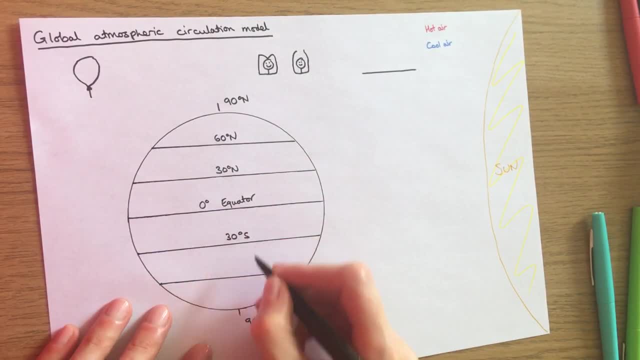 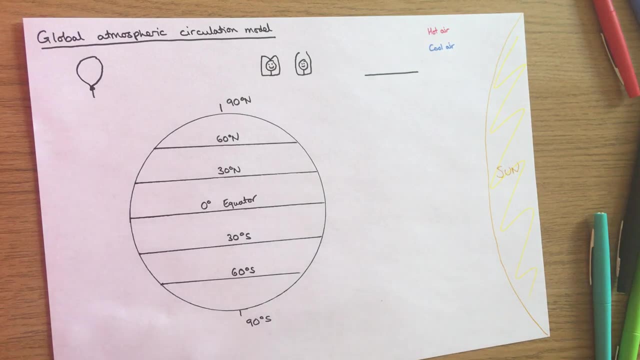 60 degrees north and then exactly the same in the southern hemisphere. So if we have a look at the sun on the right hand side, here we've got radiation coming from the sun and that enters the atmosphere. it warms the ground, that warms the air above the ground. 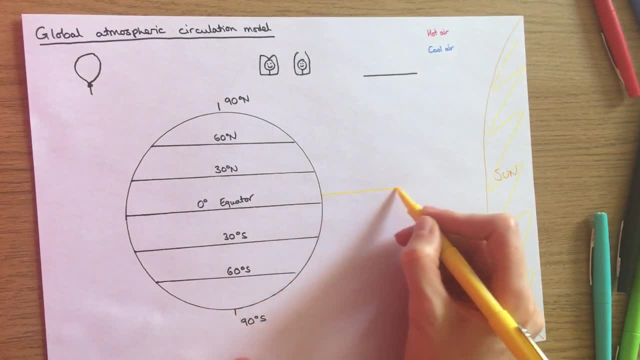 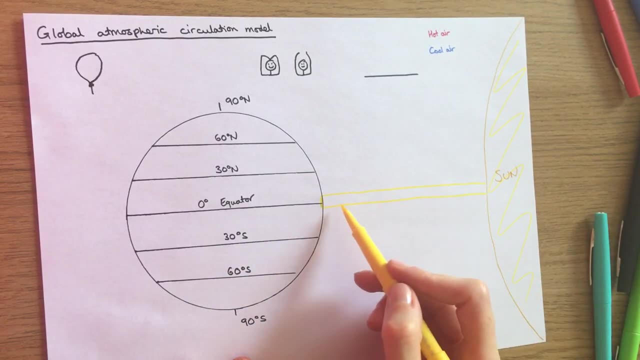 and that's why we get hot temperatures. So let's have a look at the equator first of all. Now, if this is a band of solar radiation coming in, have a look. it's coming in at 90 degrees. it's very direct. it's concentrated on just this small area. 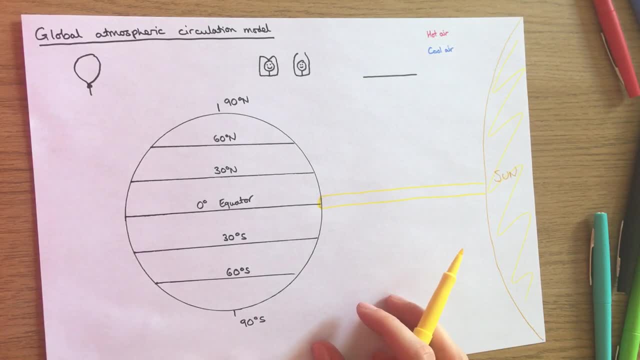 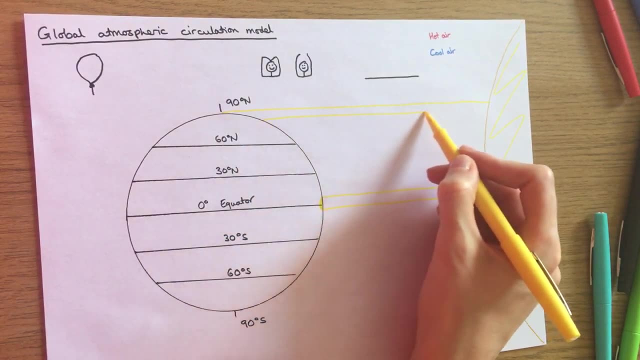 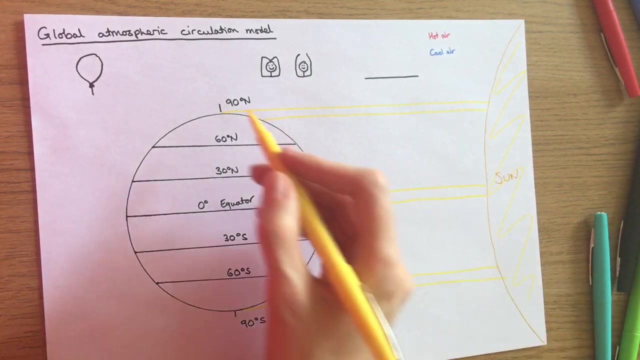 so that's why we have very intense high temperatures. Compare that now to the poles. So if we draw on the same amount of solar radiation coming in, but have a look, that same amount of insulation from the sun is spread over a much wider area. 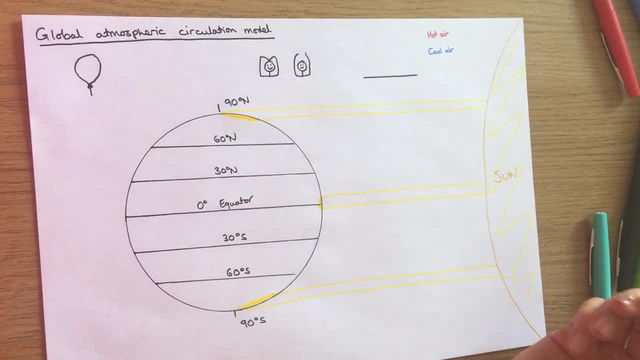 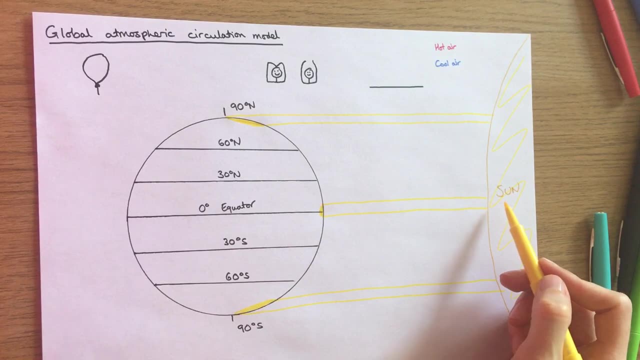 So the same amount of radiation or heat over a wide area means it's going to have lower temperatures. Now, a big misconception is that the equator is hotter because it's closer to the sun. that is completely wrong If you think about how far the earth is from the sun. this difference in 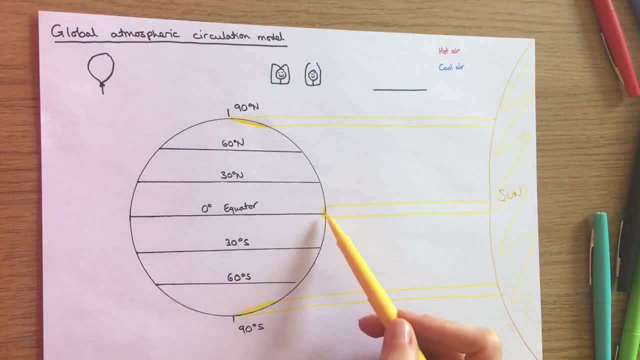 distance is insignificant. that's not the reason why the equator is hotter and the poles are colder. it's to do with the curvature of the earth and the angle the sun hits that surface. You also have more of the atmosphere which the radiation has to pass through. 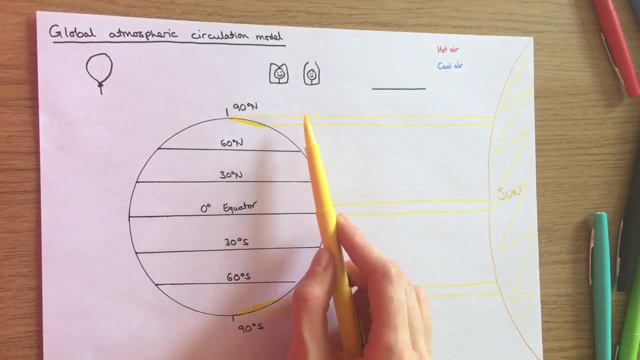 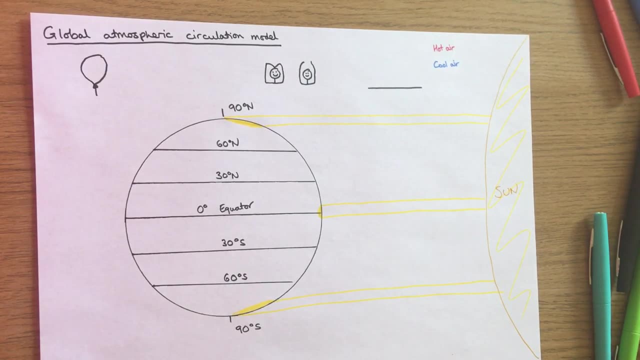 at the poles. so that means more of the radiation has to infiltrate through that layer and less reaches the surface. So that's why we have differences in temperatures. Let's have a look now at what happens to do with air movement. So we're going to have a look at the differences. 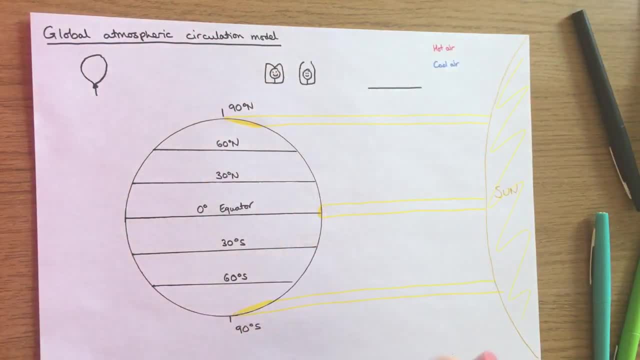 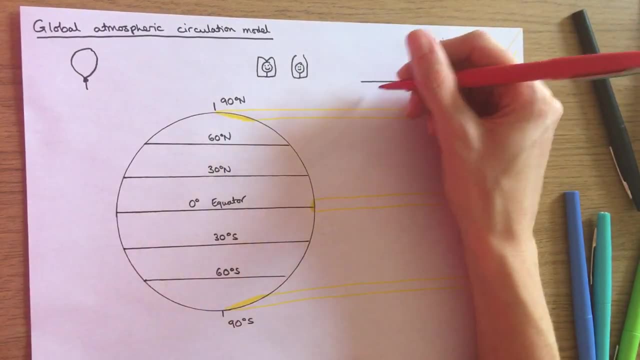 between warmer air and cooler air. So first of all, on a smaller scale, I've got my ground here. I'm going to have a look at what happens to warm air. Now, warm air warmed by the ground becomes less dense, and when something is less dense, it weighs less, and that causes it to rise. 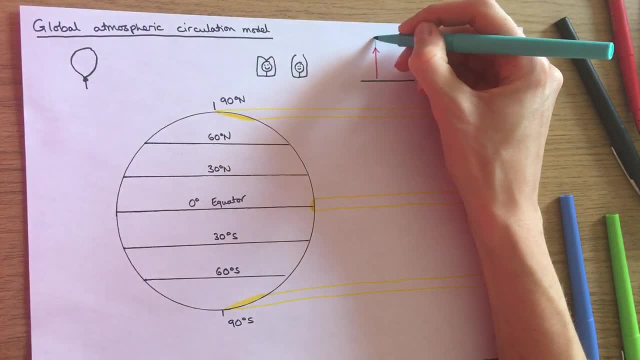 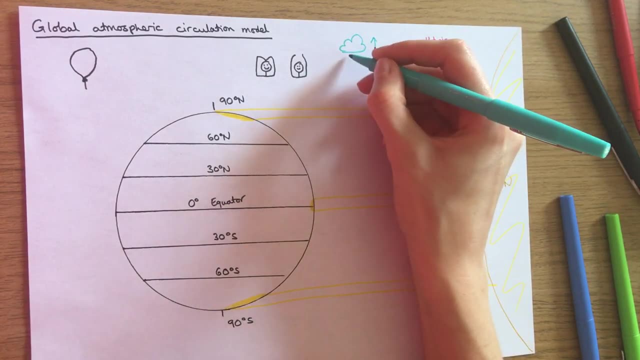 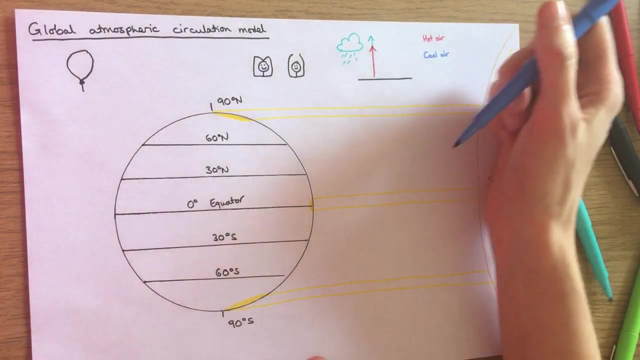 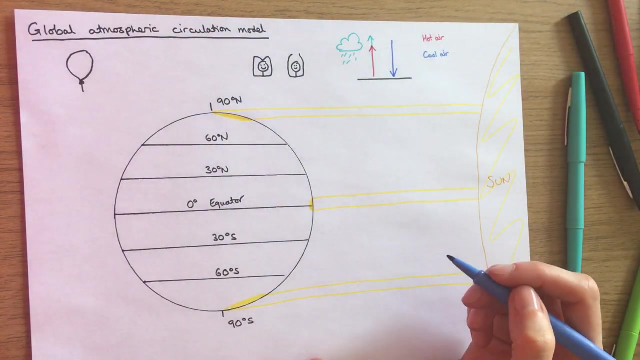 As it rises it does start to cool down, and as it cools down it condenses into clouds. If you've got clouds, you might have some rain. With cooler, colder air, it becomes more dense, So the opposite happens. So cold, air sinks. So let's just write a little summary here: So cold. 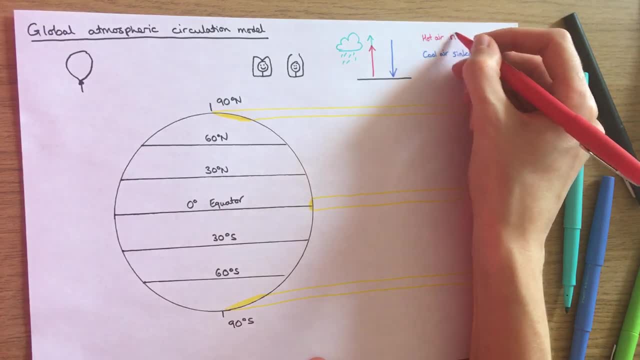 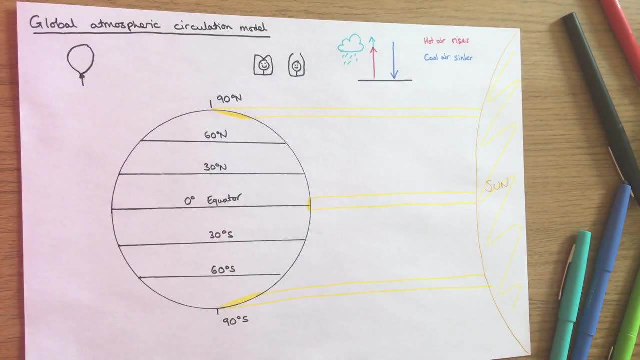 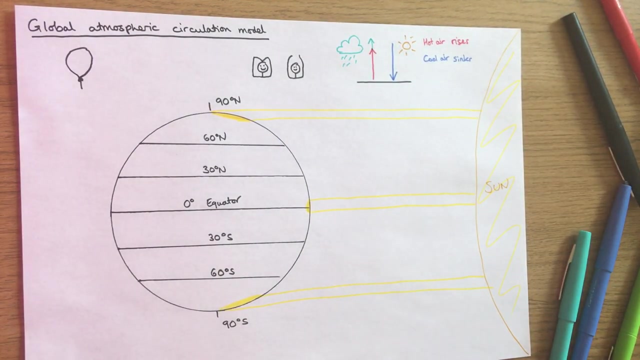 air sinks and hot air rises. Now, when we had hot air rises, we said it was condensing and forming clouds. But if the air is sinking, that doesn't happen. So when we have sinking air, we have quite clear conditions. Okay, So let's link this into the idea of air pressure. 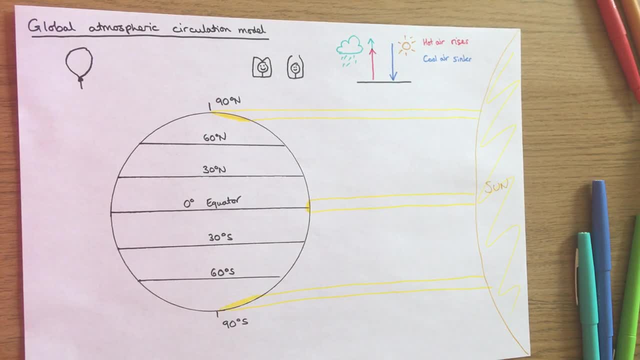 because we don't really think of the air as weighing anything, but it's pressing down on the surface And that has a huge impact on our climate and our weather. So I'd like you to have a look at my little stick pen here. I'd like you to put your hands on your 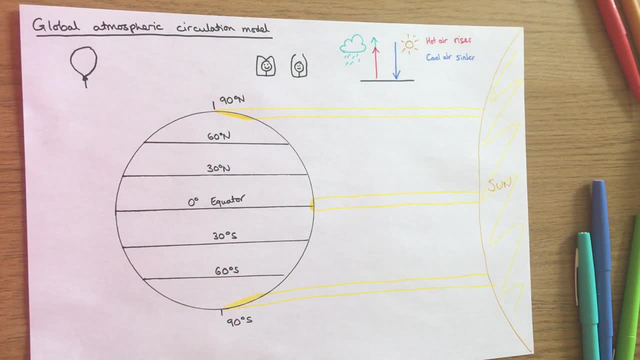 head like this one here And you can feel your head probably feels quite heavy. You've got the pressure of your hands weighing down on your head. Okay, you're not going to raise your hands up like my second stick man here. So we've. 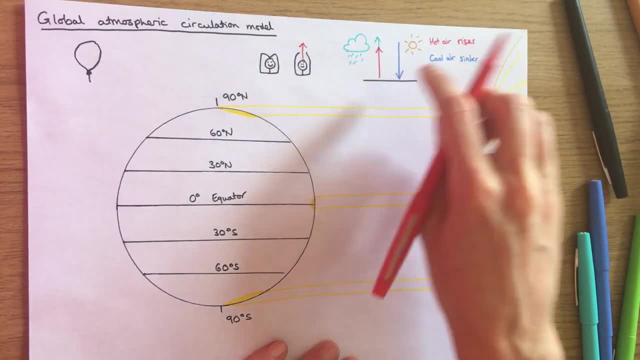 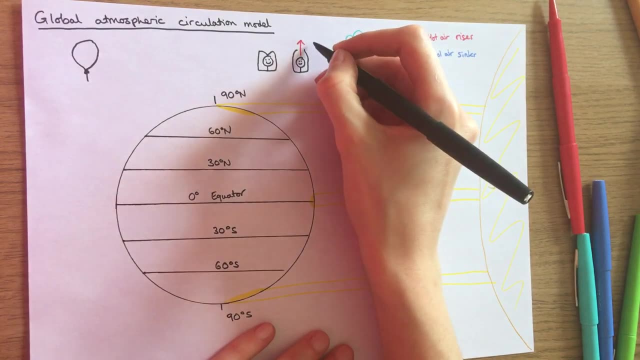 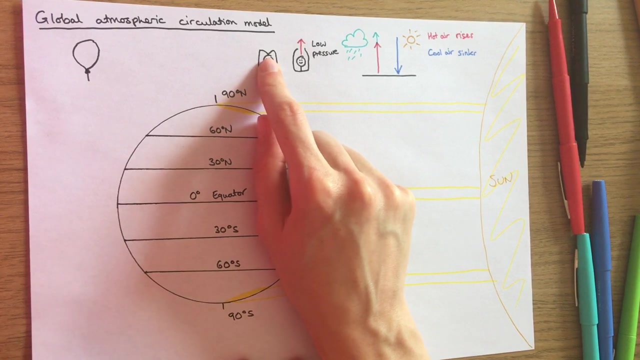 got that rising of your hands, just like our air rising, And here your head feels very light. it has no longer got that pressure of your hands pushing down on it, So here we have low pressure. Okay, you're now going to bring your hands back down and press them. 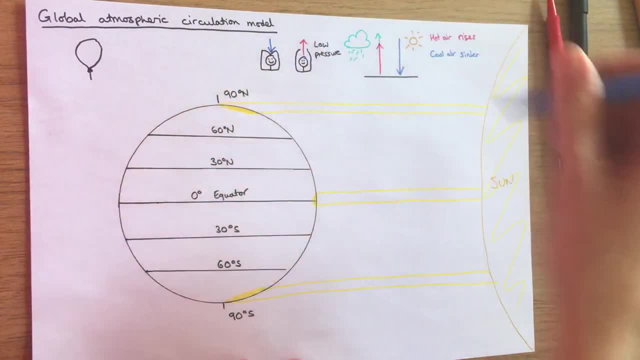 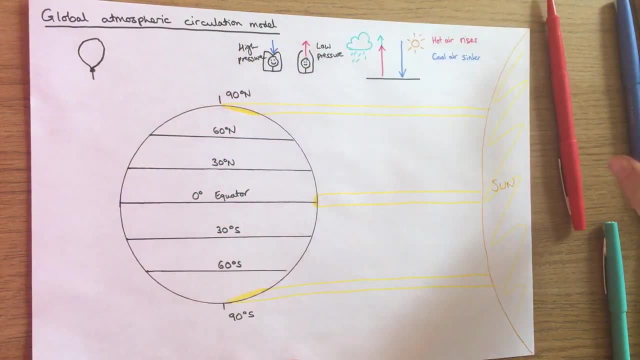 on the top of your head, Just like our sinking air. you're feeling that pressure again. Okay, so we're in high pressure in our rotator cuff now. So let's just summarize that here: hot air rises equals low cold air sinking equals. 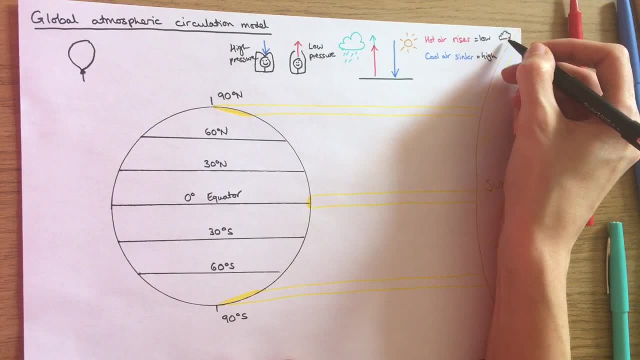 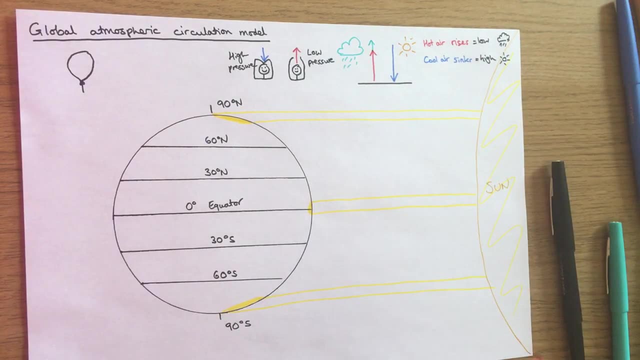 high pressure and just to remind ourselves: low pressure: we have our clouds and rain. high pressure: we have quite clear conditions. So let's keep that in our mind. We can refer back to that as we go through, because we're going to have a look at that on a larger scale. 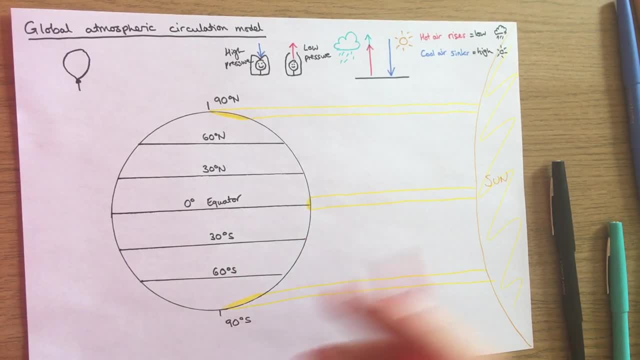 on a global scale. So let's start with the equator. we know it's very, very hot there and we need to just keep our seeking ages aligned to our low pressure and AIaya, And there the economies will occur. We can see a le Crystal Arrider taking off from a big obsinary, And that's just my clicking that we've got on there. It's very sharp. We might 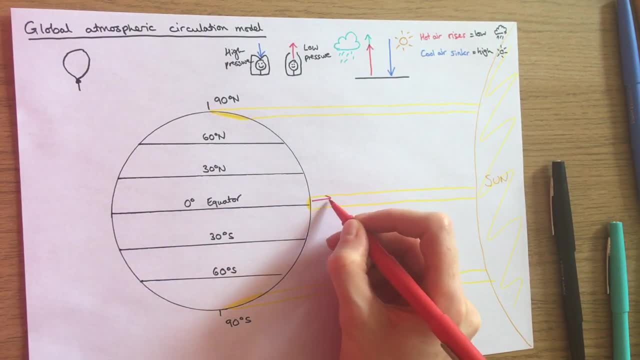 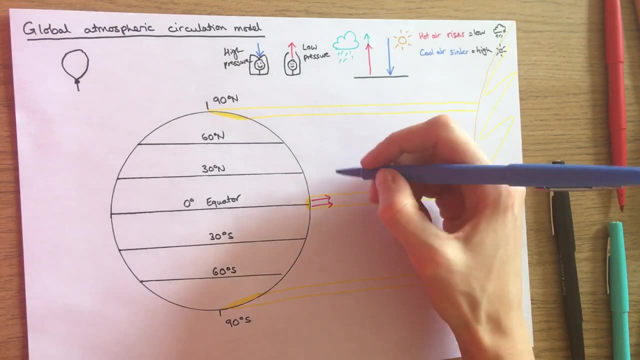 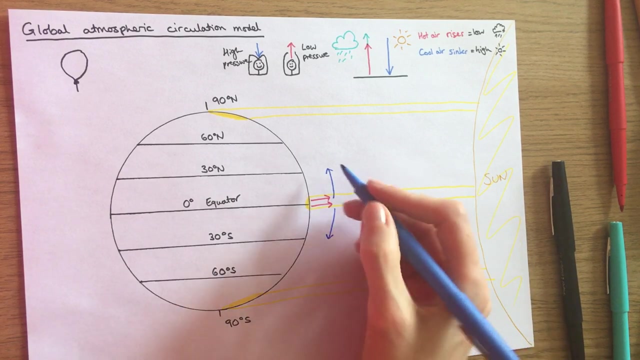 we know if we've got hot air, it's going to rise. so let's draw our arrows in now. as that air rises and gets further from the earth's surface, it cools. it also moves away from the equator, so our cooling air is moving away. and then, when it gets, 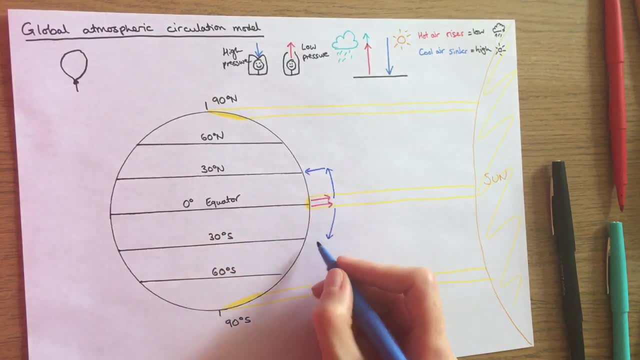 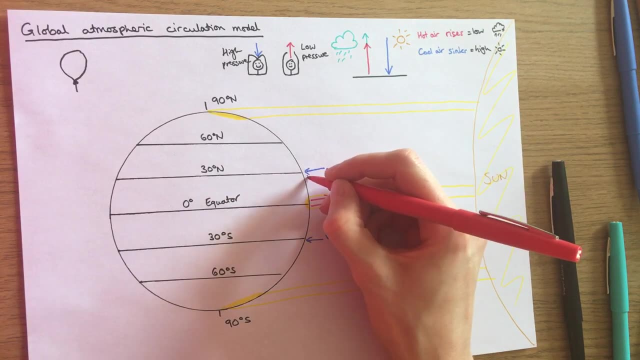 about 30 degrees north, it begins to sink. let's draw that on and then, as it's nearer the surface again it's got lots of sun's radiation. here. it's very warm, so it's going to heat and we can see there. we've got a cycle going on. now we 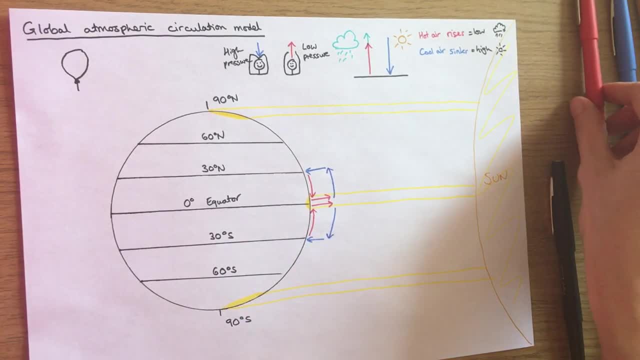 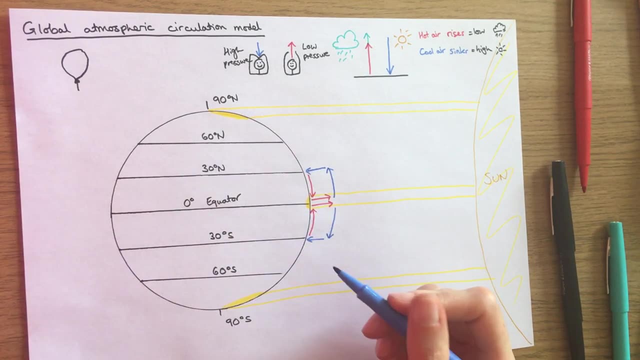 call this a cell. so let's have a look at the poles as well, because you know what the conditions are like in the poles. we know they're extremely cold. so if we have a look, cold air sinks, so let's draw our arrows on showing off sinking air. 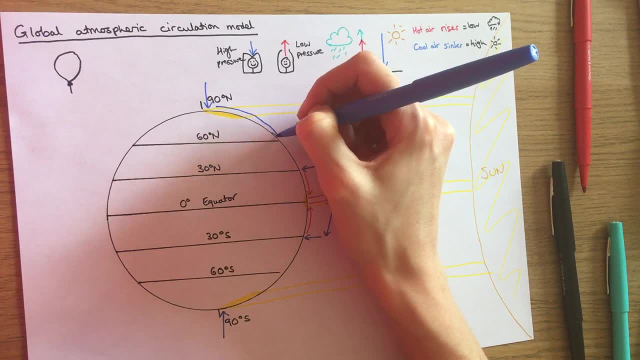 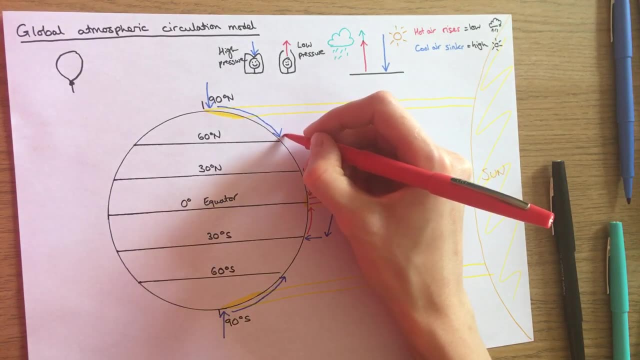 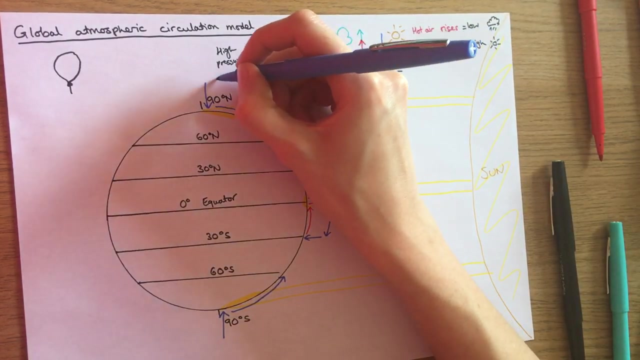 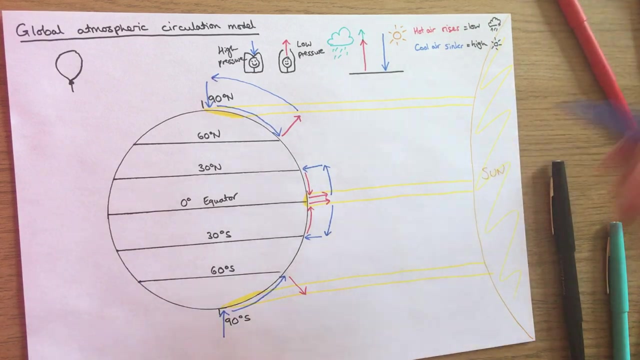 now. the air is still quite cold here, so let's keep going. keep this in blue. and moves round to about 60 degrees north and then it gets warmer here. so the air warms and rises and cools again and moves over. so we've got another cell forming there. it's exactly the same in the southern hemisphere. 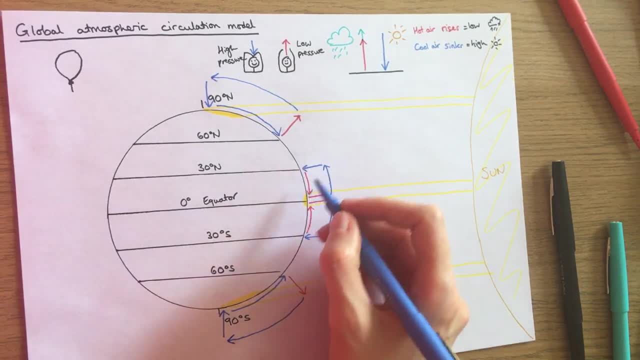 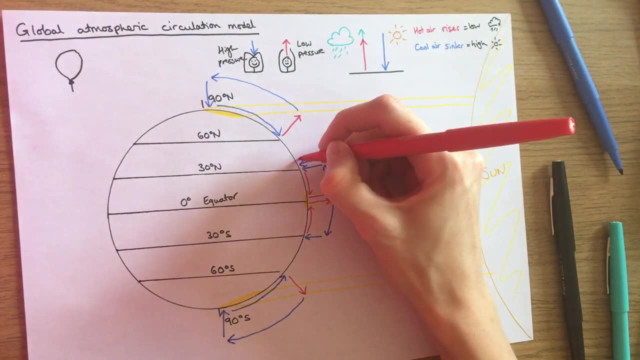 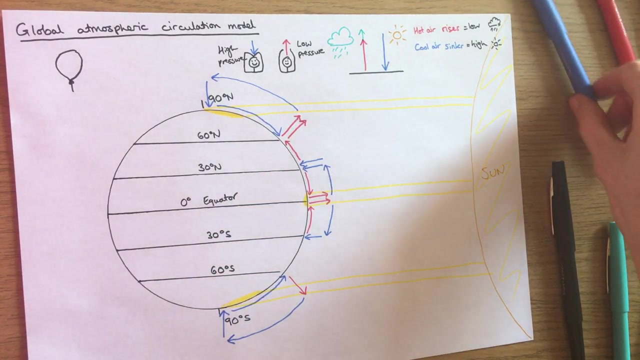 okay. so what's happening in between? so let's have a look here, on the 30 degrees north, we had our cold air sink here, so that's, that's the same. here, that air is going to warm as it's warming here, it's going to rise again. it's becoming less dense and then, to complete that, 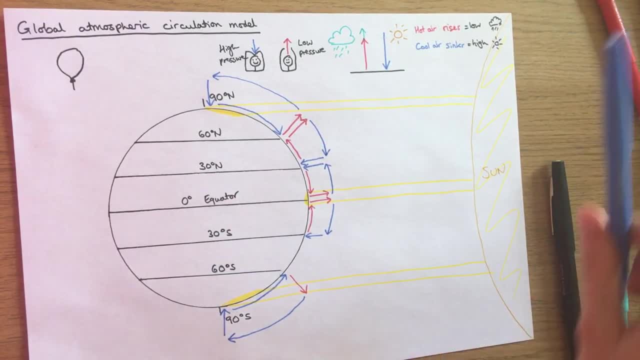 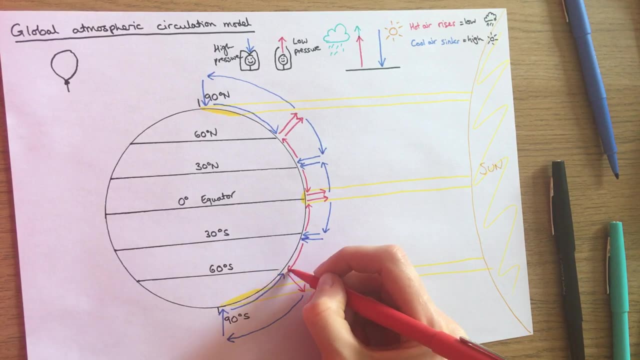 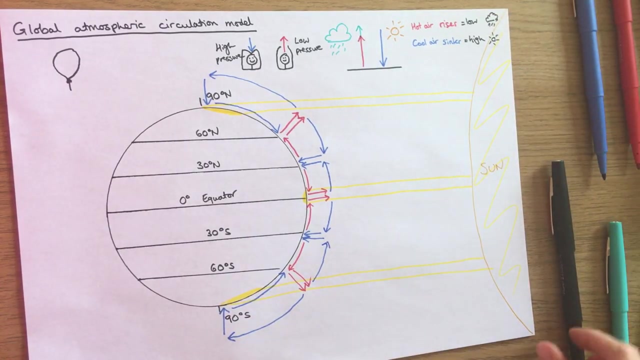 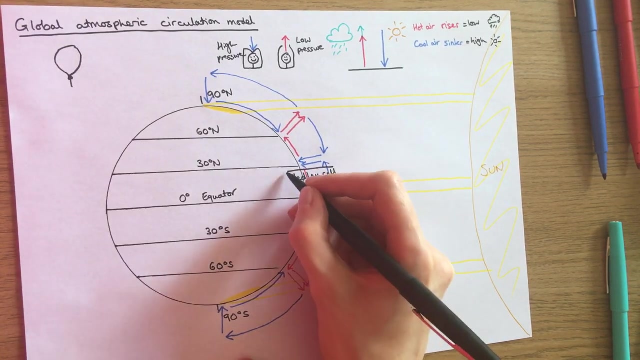 cycle. the air is going to move back towards the equator. okay, it's exactly the same in the southern hemisphere as well. so this is what we call the tricellular model, because we've got three different elements that move in a cells forming here, so let's label them up here. we've got the Hadley cell. this: 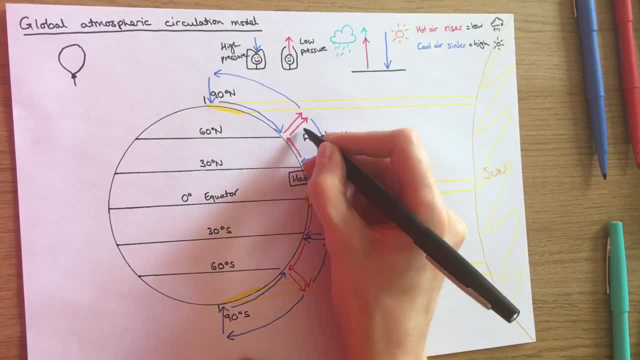 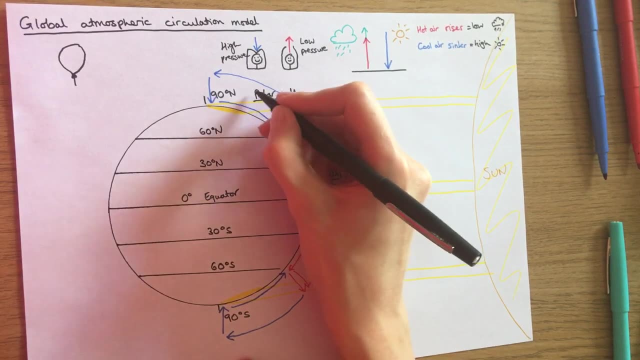 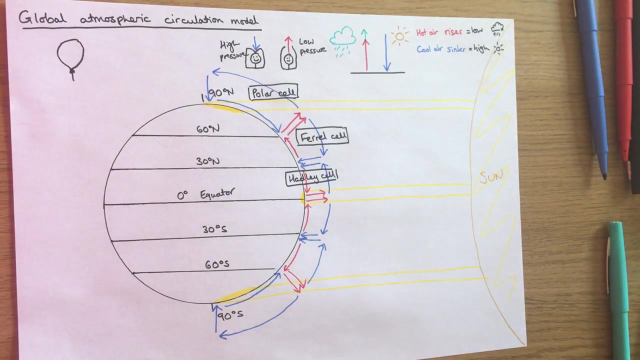 one is the ferrule cell and this one is the polar cell. okay, so we've had a look there at how the warming and cooling air moves and the patterns formed there, but we need to know why this is important for geographers. why is this? why do we? 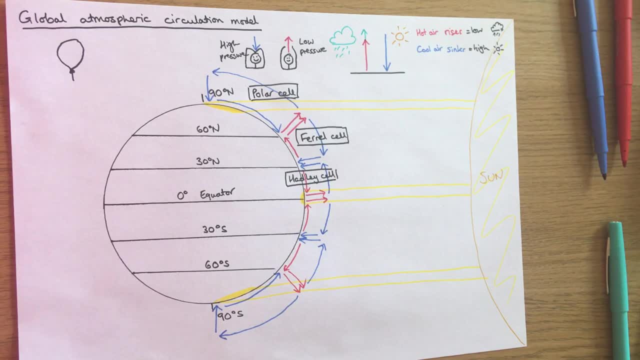 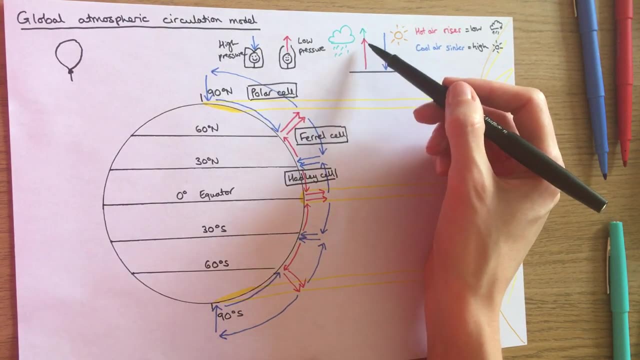 need to know this. so it's all to do with the different conditions we find there. so let's start at the equator again. now we've got our warm air rising and we said: when our warm air rises, we get condensation as the air cools, and then 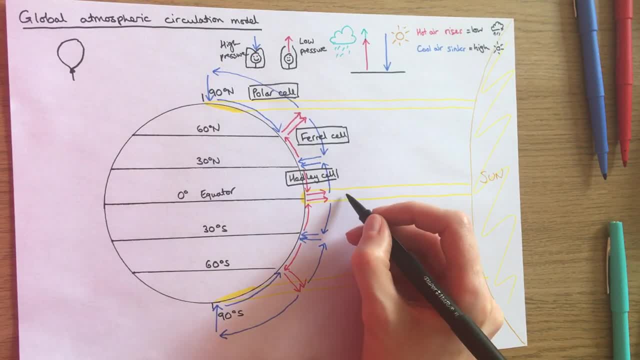 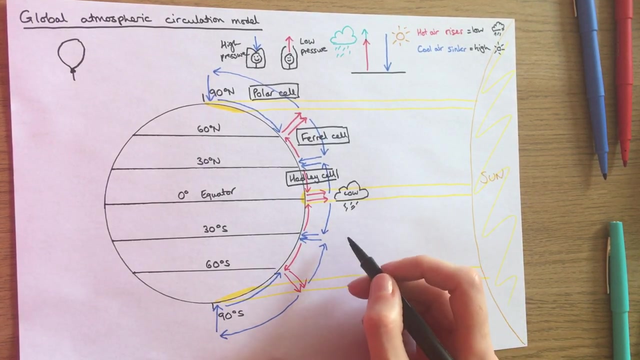 clouds form and we have low pressure there. so let's draw that on. so we've got our cloud. it's low pressure. we've got rainy conditions, you- okay, let's have a look next at 30 degrees north and south. so here the air is sinking okay, which means you've got high pressure. we said that's quite clear. 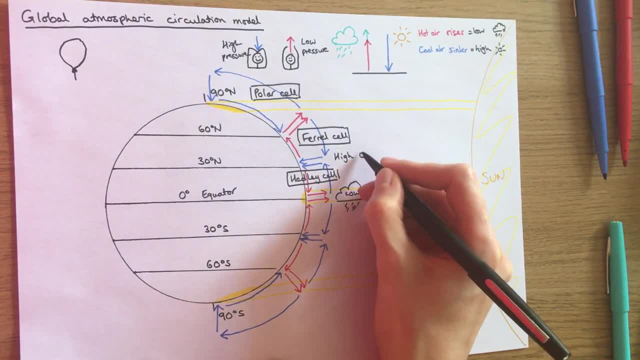 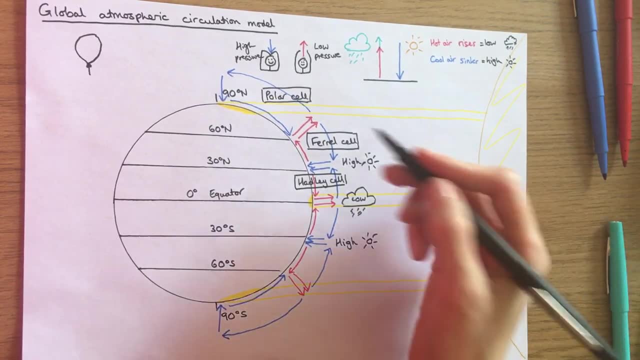 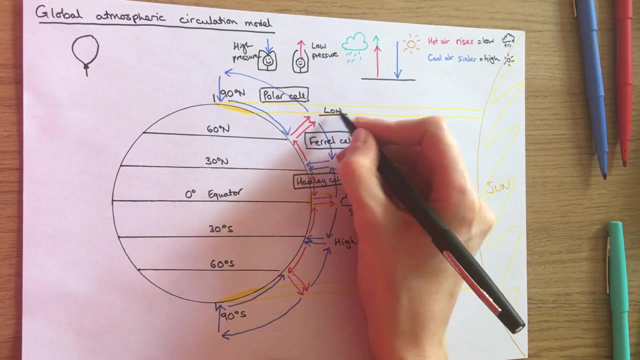 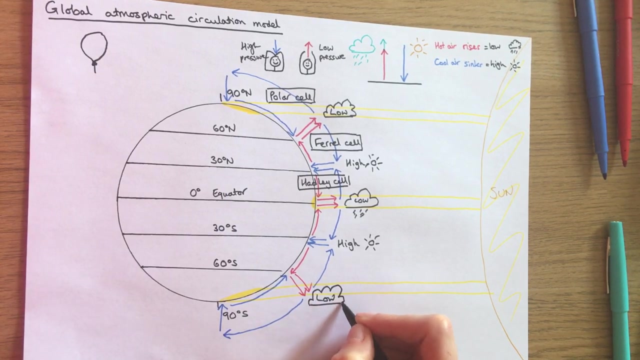 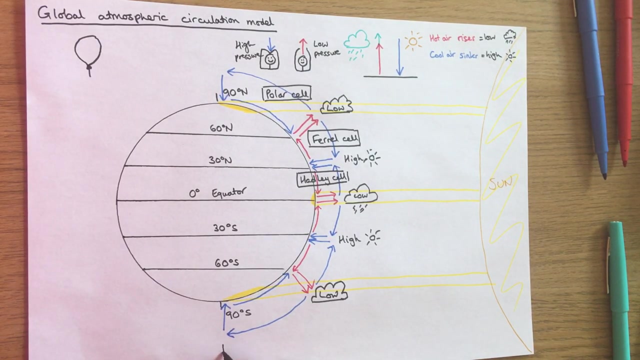 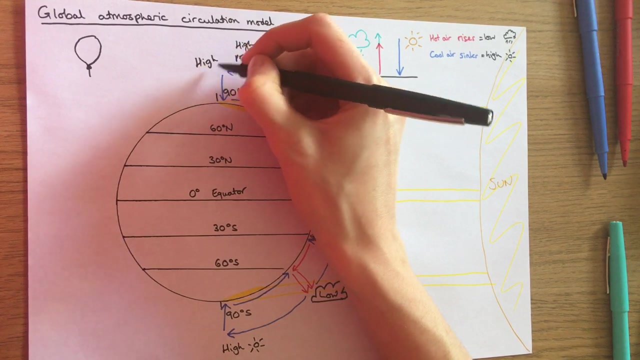 conditions- okay, let's label that on, and the same in the southern hemisphere. okay, the next bit. we've got warmer air rising, so again, low pressure, challenge, clouds, rain- really imagine this. energies from the sky, clouds, rain. and then finally, at the poles, we've got Kita. 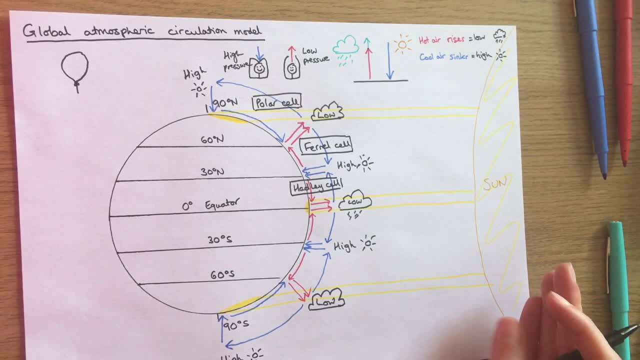 sinking air or high pressure. now I put the sun here. obviously, in the winter months there is no sun, but it represents clear skies and not much precipitation in this case, so we know what the conditions are like we it's going to have. Now, as geographers, we can tell what kind of biome you might. 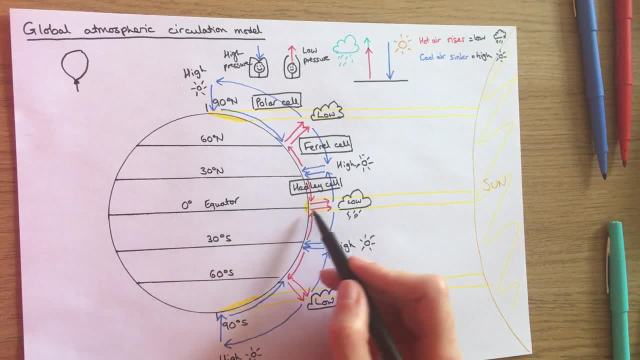 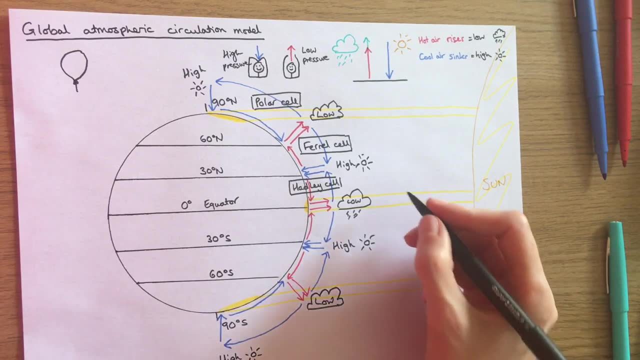 find there as well. So let's start again with one. we're familiar with the equator. We've got very high temperatures, as we mentioned, and we've got low pressure, so we've got lots of rainfall. So very high rainfall and hot temperatures. Now what? 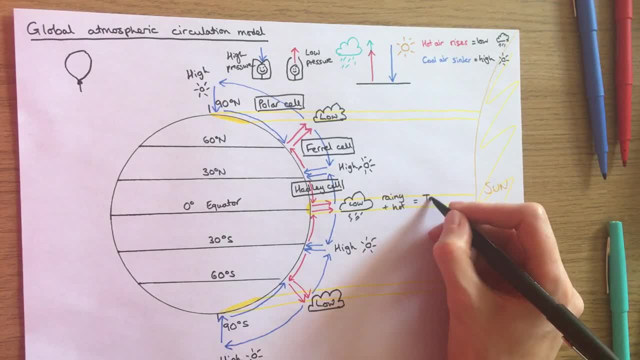 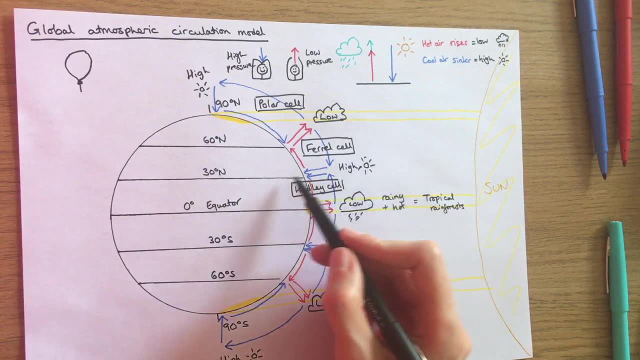 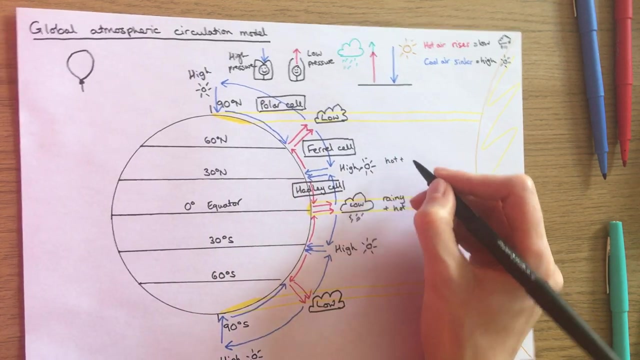 type of ecosystem likes those conditions. So here we find the tropical rainforests. Okay, moving to 30 degrees north. So here it's still very hot. we're still close to the equator, so it's hot, but because of the high pressure we haven't got that. 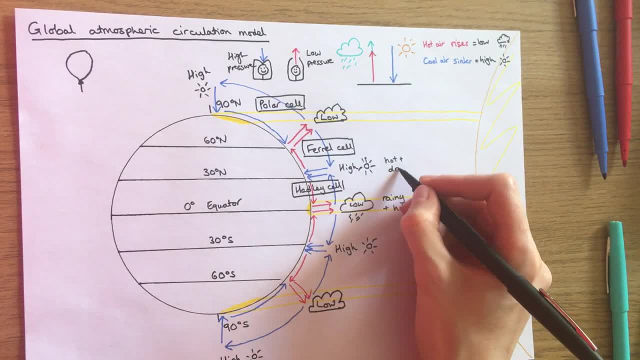 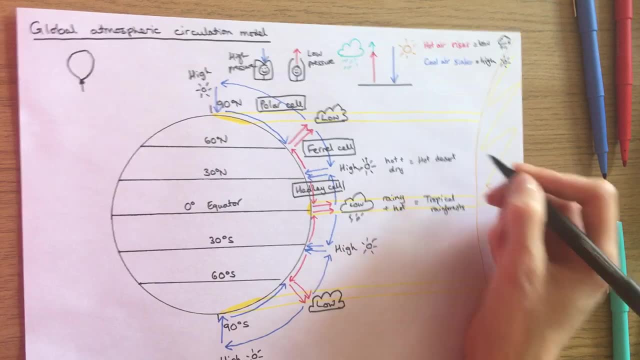 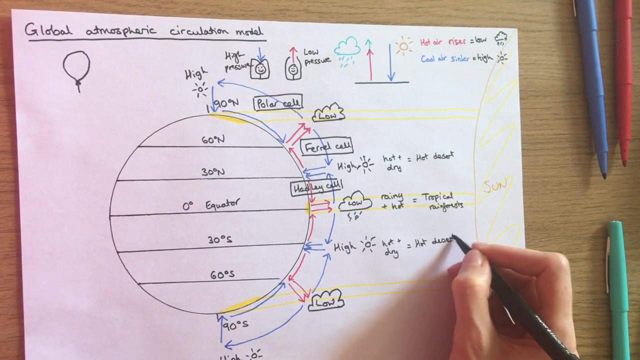 condensation and clouds forming. We've got clear skies. it's very dry. So what would a hot and dry ecosystem be? It would be a hot desert, So the Sahara, for example. Okay, let's have a look at the pole. So we've 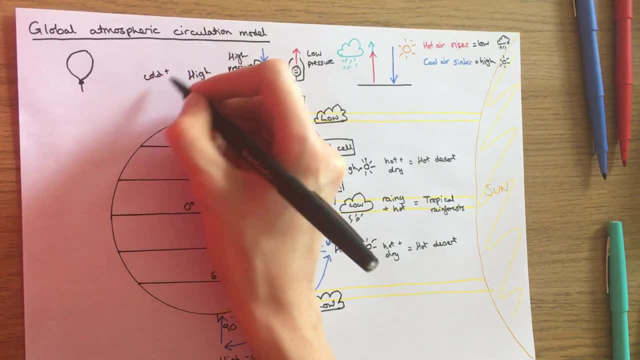 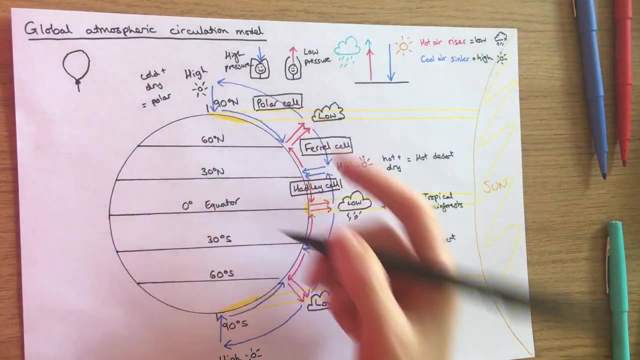 got the Sahara and we've got the desert. So we've got the Sahara and we've got the, got high pressure, we know very cold temperatures. so again it's cold and it's dry. so here we've got our polar regions, so our arctic regions in this case, and antarctica here in the bottom, so cold. 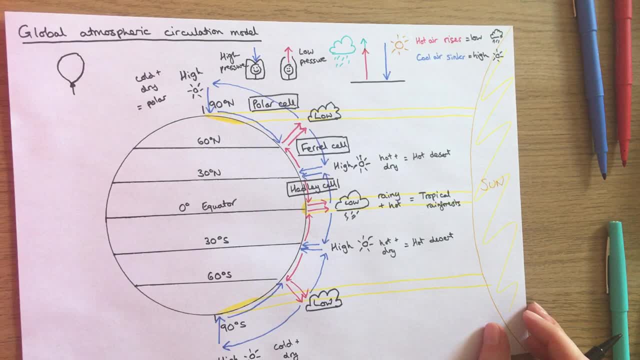 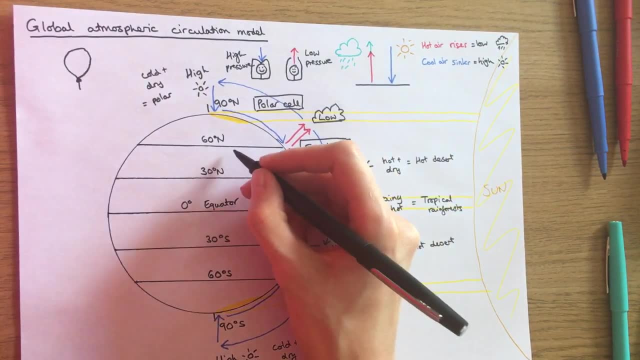 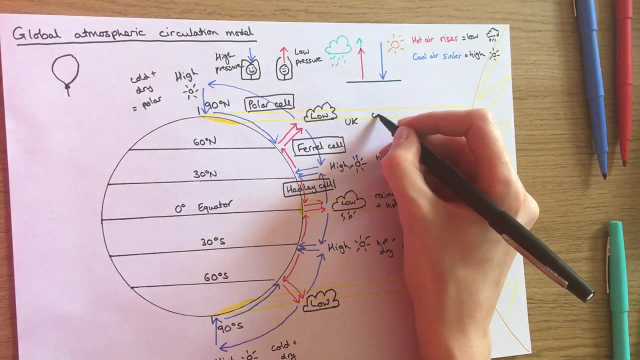 and dry. so look at that, we've got the movement of air, we've linked it to the conditions of the climate and we've linked it to different biomes. you know, and just looking at 60 degrees north, the UK is close to this particular line of latitude, so here it would be cooler and rainy. 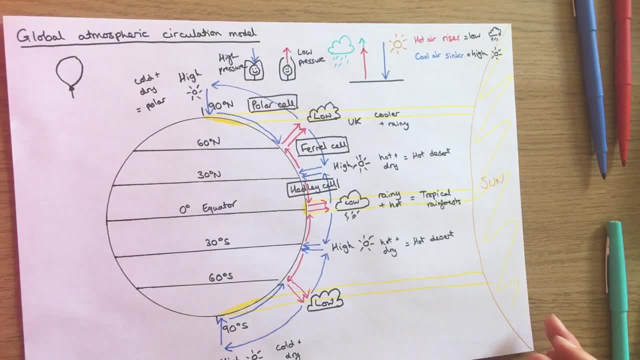 so you've got the example of the UK there. okay, let's have a look at the next part, which is to do with wind. so I'd like you to have a look at my balloon I've drawn here. now, imagine you blow into a balloon, you squeeze all that air in. they'd have lots of high pressure and the air pressure is. 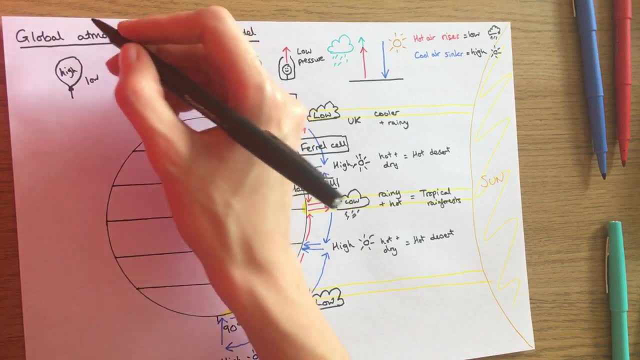 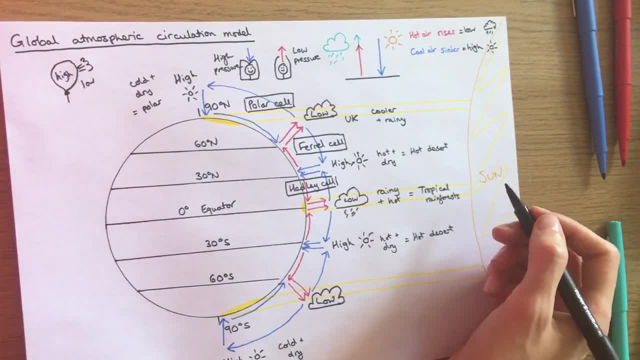 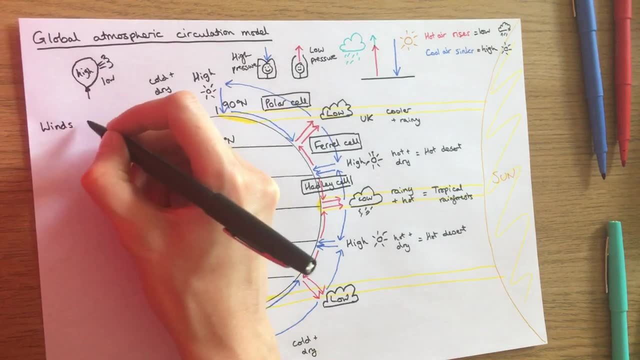 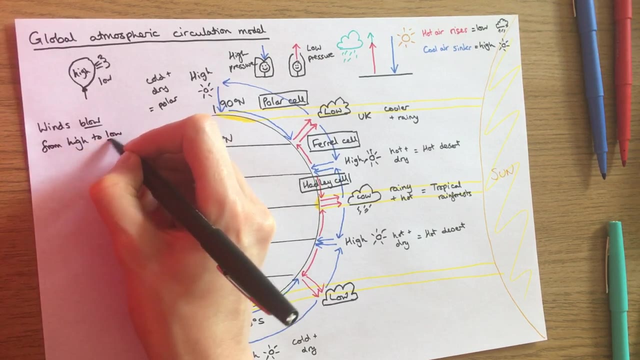 in the side. all that air would rush out, because air moves from high pressure to low pressure. to try and balance out, it's got a little rhyme for you. the same happens with winds, so winds blow from high to low. so how's that working on that? well, we've got high pressure in the poles and 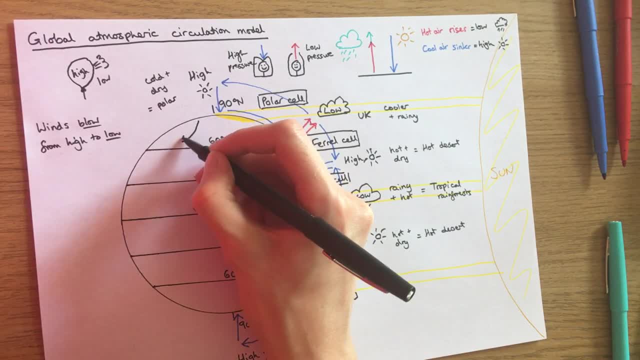 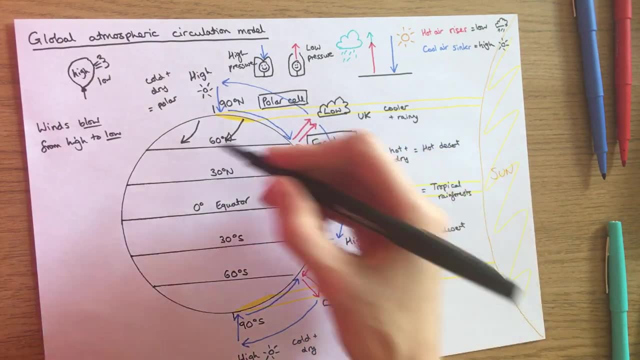 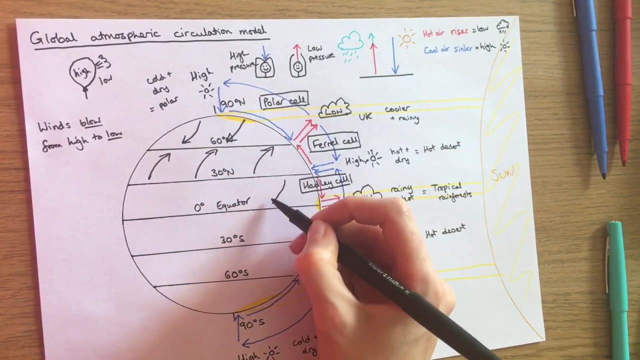 we've got low pressure at 60 degrees north, so our winds blow from high to low. the next bit: here we've got low pressure, here we've got high pressure, so it's going to be the opposite direction, and then again from high to low. now you might be looking at that thinking, well, Miss Simpson's drawn some really curved wonky. 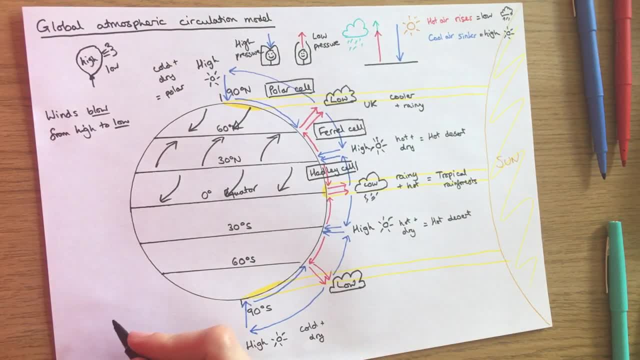 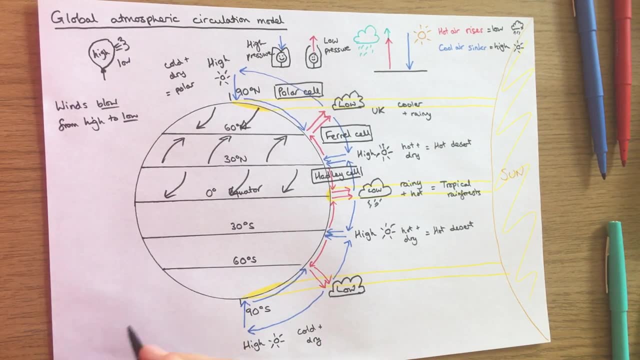 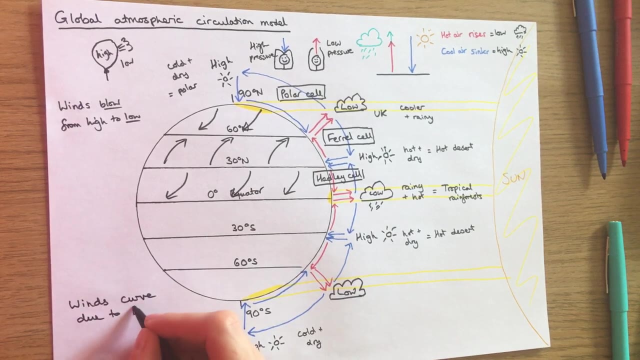 lines there? I haven't they. they are correct because the earth's rotation, the spin of the earth, causes those winds to bend and we call that the Coriolis force. so let's just jot that down. so winds, Coriolis force, curve due to the earth's spin. 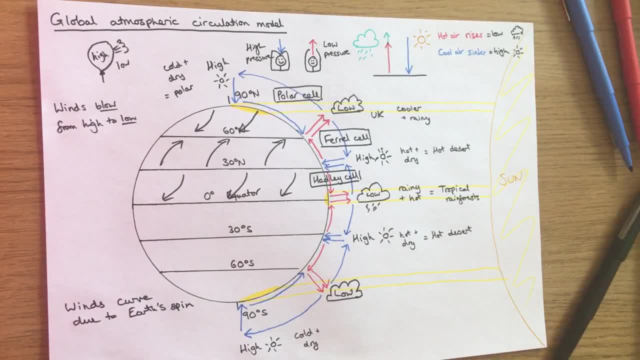 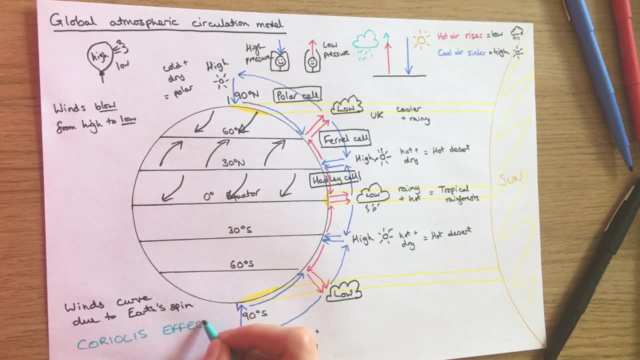 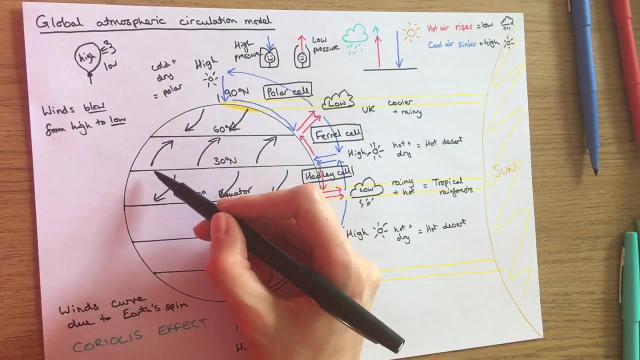 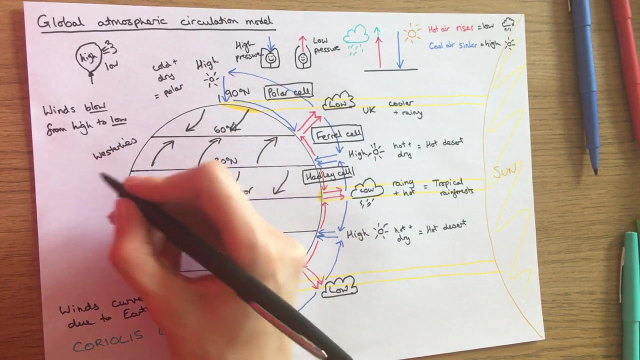 and that really good key term was the Coriolis effect. okay, um, final thing to add on is the name of these winds. so we name winds from where they come from. so these ones here move from west to east. we call them the Westerlies, and these are. 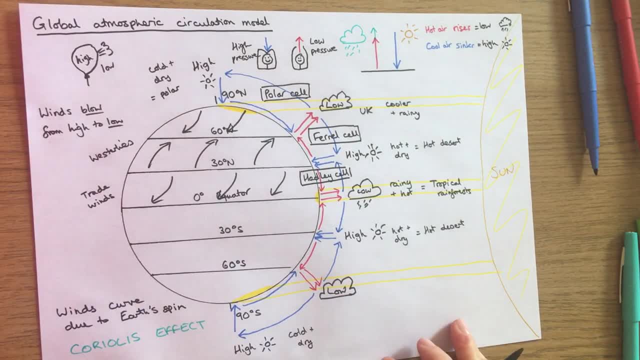 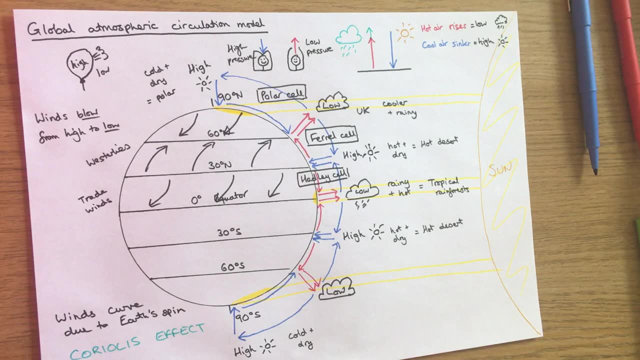 called the trade winds. Okay, I hope that has been helpful talking you through and explaining the global atmospheric circulation model. Thank you very much for your attention.